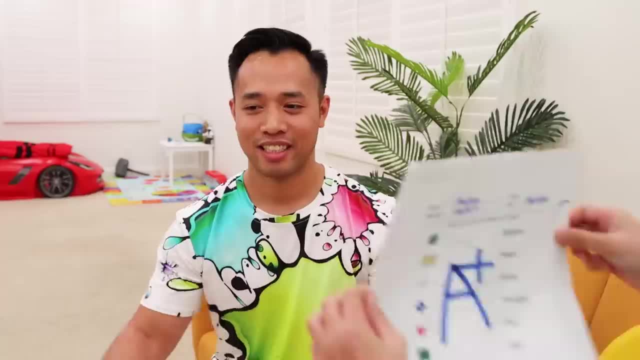 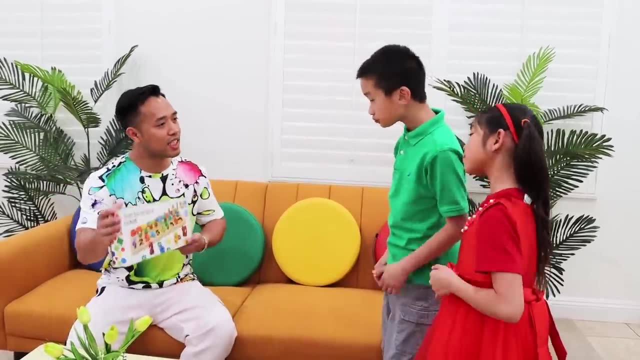 Uncle Jay. Uncle Jay, Check our grades. Good job guys. Huh, Who's a big A? Sorry, No, don't cheat again. guys Here, Study with this. This will help you with shape and math. What shape is this? 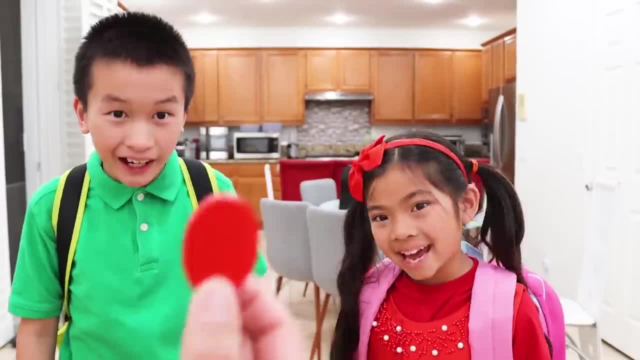 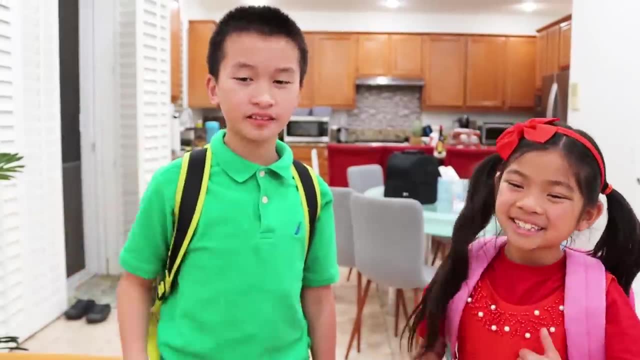 Uh, This is A oval. It's shaped like an egg. Okay, What shape is this Rectangle? No, guys, This shape has a heart, Like this Garden. What shape is this Star? No, guys, It's a triangle. 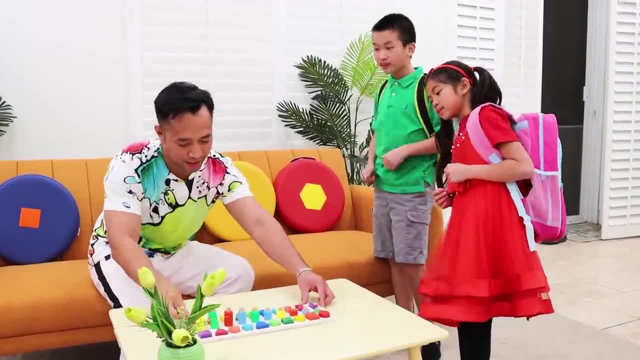 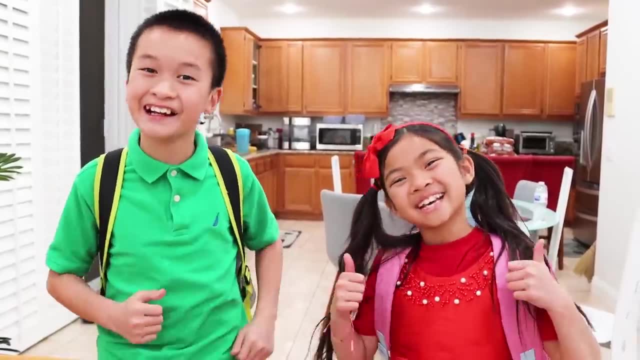 It has three sides, like a pyramid. Oh, Let's learn math now. One plus two equals three. One plus two Two equals three. Good job, guys. What's two plus three? Ah, four, Six. No, guys, The answer is five. 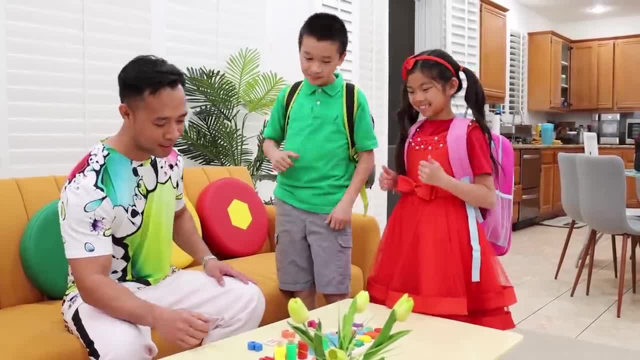 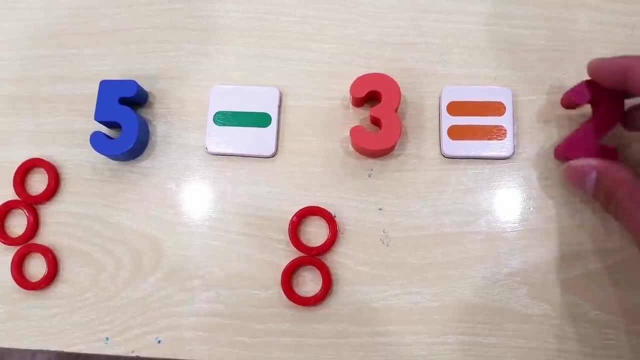 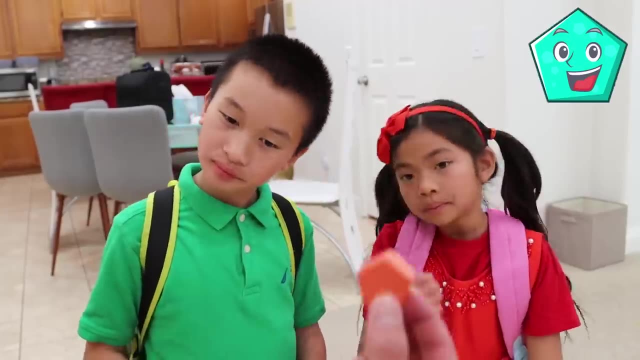 Oh, Can you help us with subtraction, Of course? What is five minus three? Oh, that's easy. Ten, Twenty-one Five. take away. three equals two. Four plus five equals nine. Star Pentagon. Remember to study hard, okay. 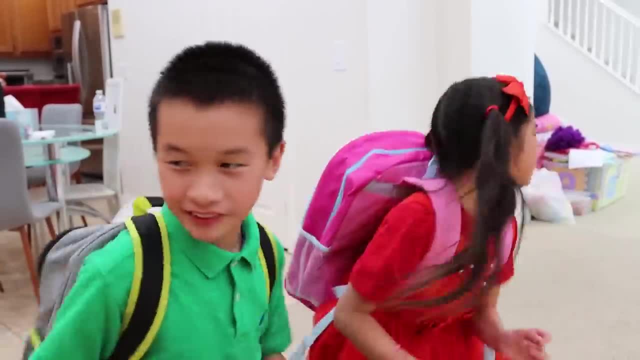 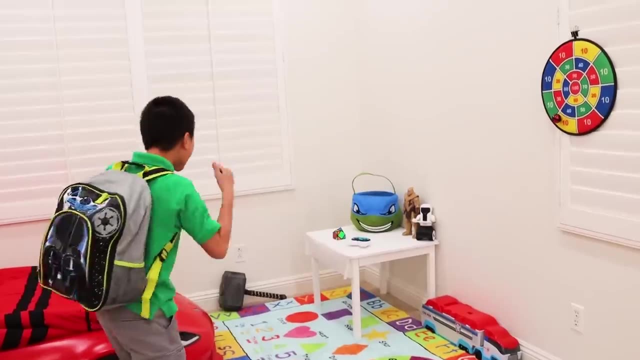 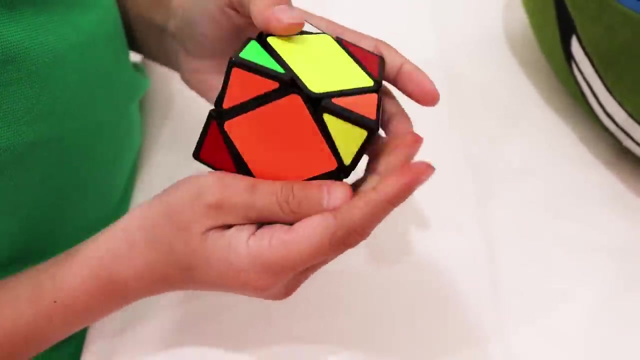 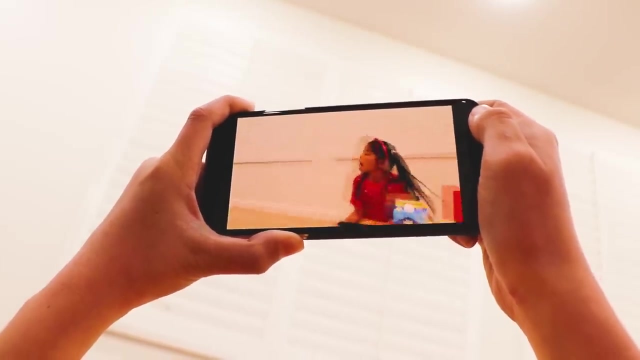 Okay, I'm going to go study, Study. I'm going to play games. Let's play this game. Yeah, Rubik's Cube Con. I'm going to watch some videos before I study. I love these videos. I can watch them all day. 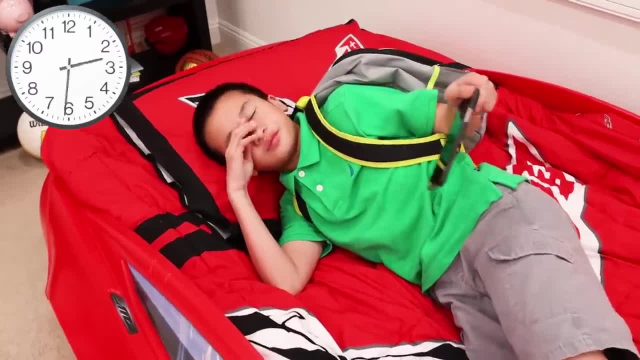 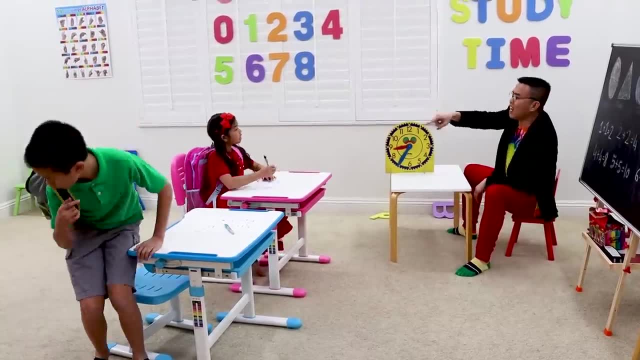 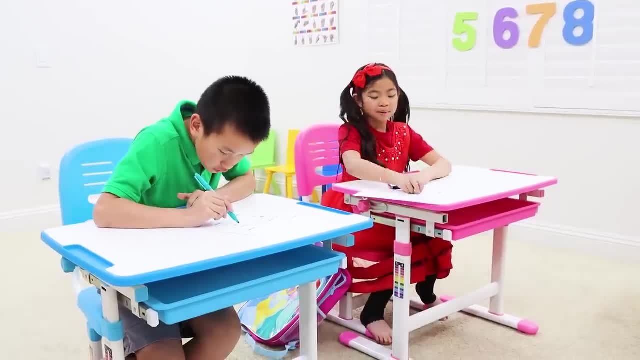 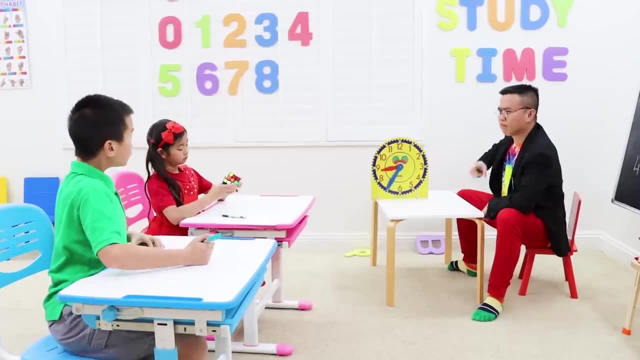 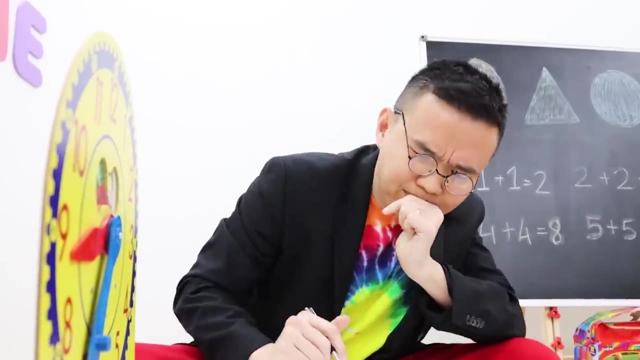 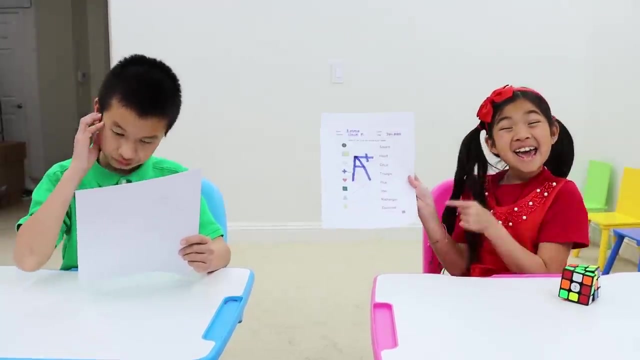 This is so hard. I'm done, so I can play with my Rubik's Cube Time's up. Oh, no, To your taste, guys. Thank you. I got an A. I got a C. Remember to always study Bye. 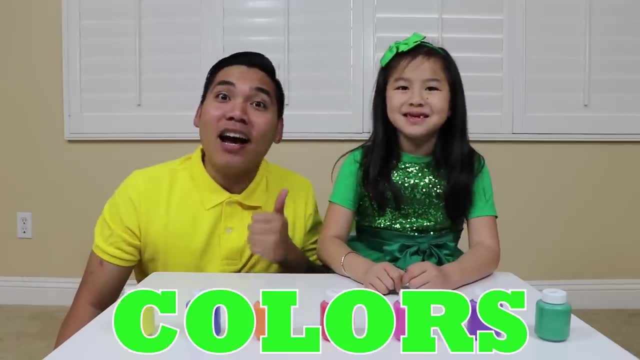 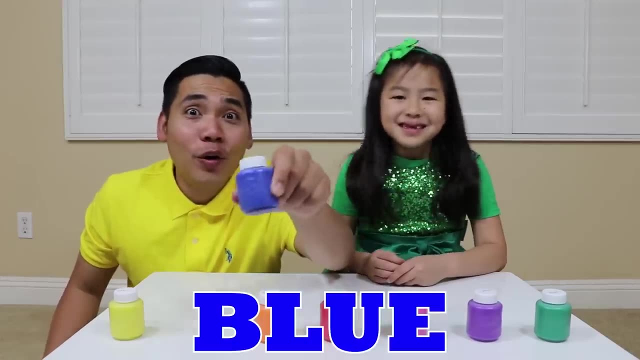 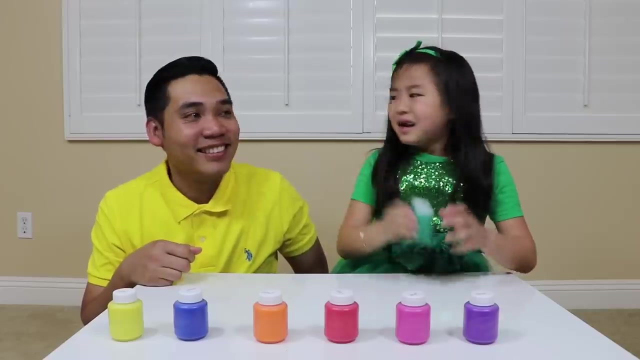 Hi guys, Today we will learn about color, animal and fruit. Wow, Look at all the colors: Yellow, Blue, Orange, Red, Pink, Purple And green. Let's do some magic painting, Uncle John. Okay, Can you paint my hand green, Uncle John? 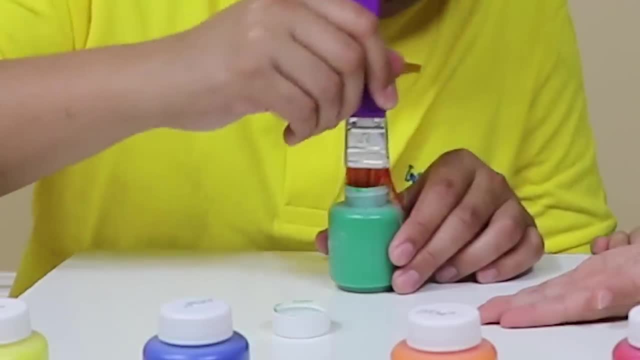 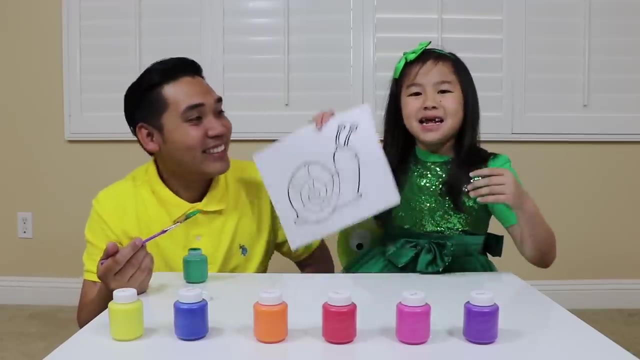 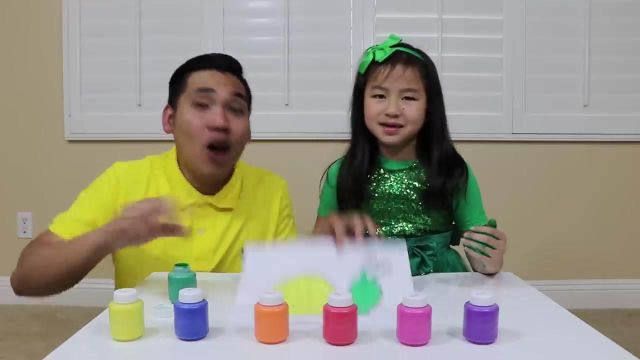 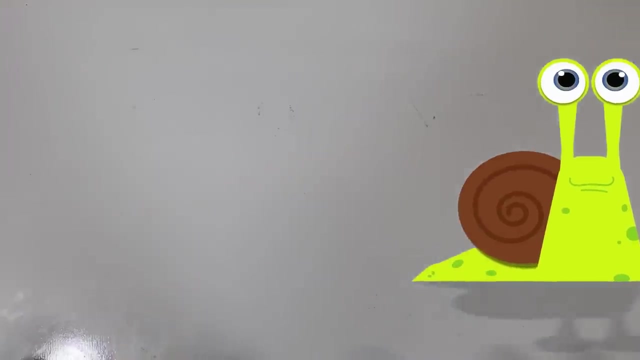 Okay, Let me do it Green. Now I will paint the snail green. Wow, Check out Jenny's snail guys. It's green and it has a yellow shell. Wow, That's so cool. I will do it on your hand, Jenny. 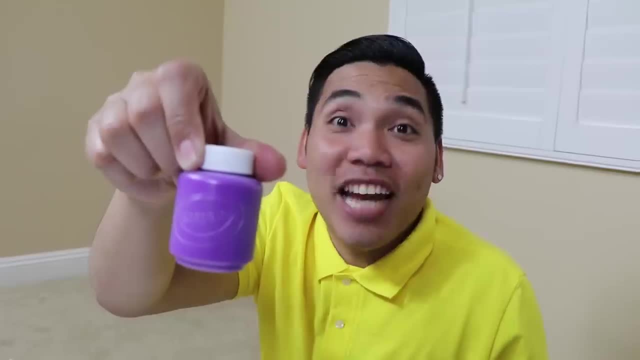 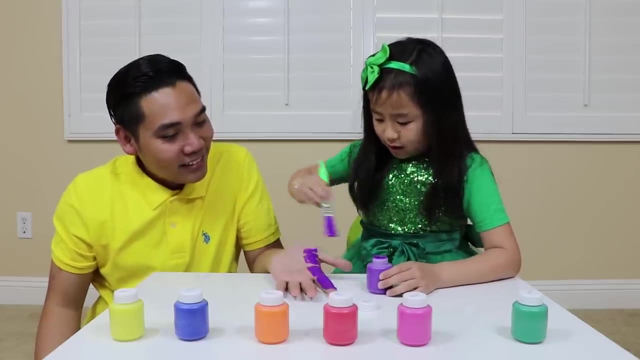 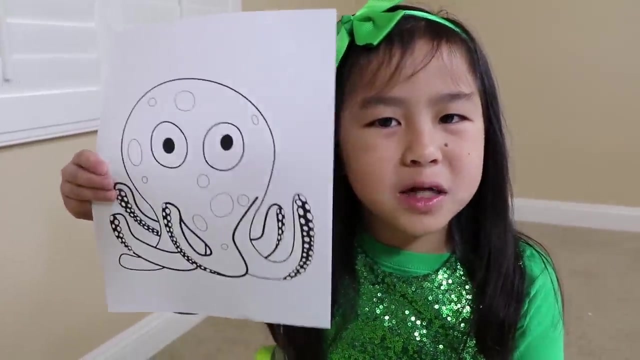 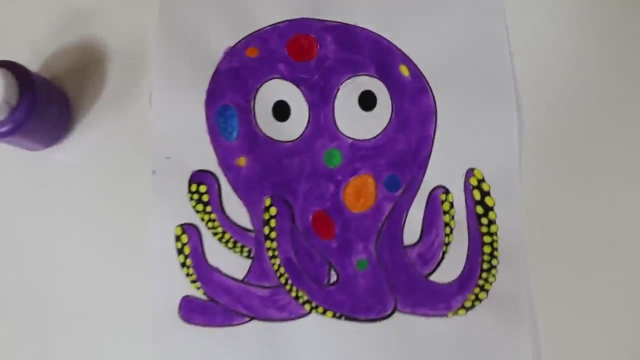 Yeah, Hmm, I will choose purple. Jenny, can you paint my hand? Okay, Here you go. Purple. Uncle John, paint the octopus purple, Okay, Jenny. Wow, This is a cool purple octopus. guys, I'm going to pick the color pink. 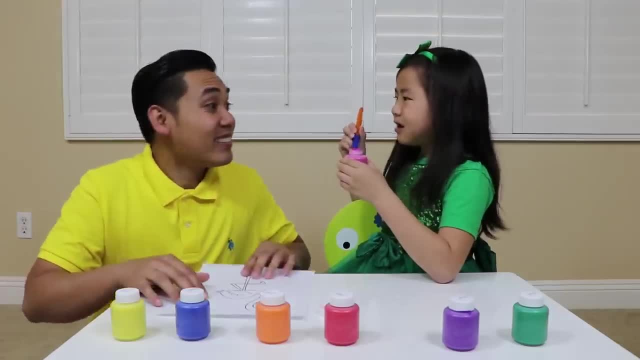 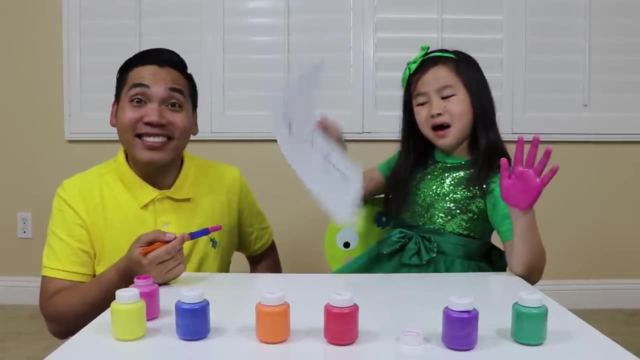 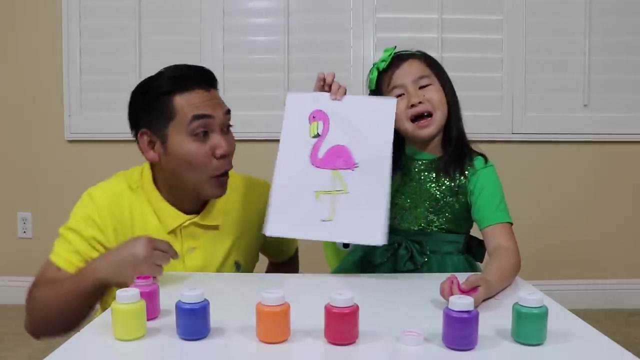 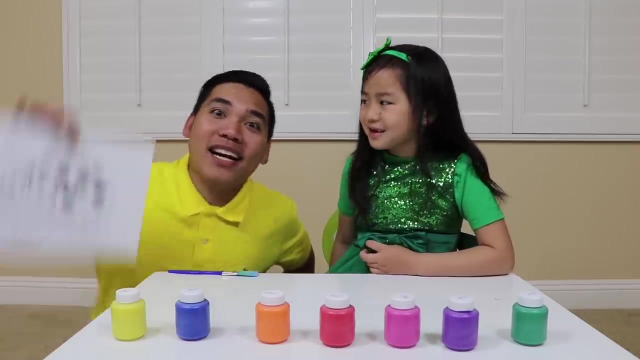 Okay, paint the flamingo pink. Jenny, Can you paint my hair uncle? Okay, Pink, I'll paint the flamingo. Check out my pink flamingo guys. Wow, awesome guys. Now I will paint the ladybug with the red color. 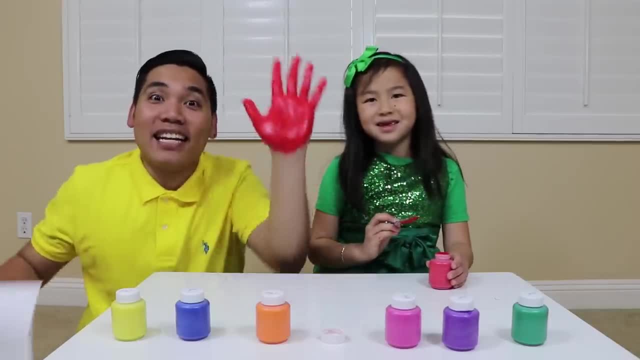 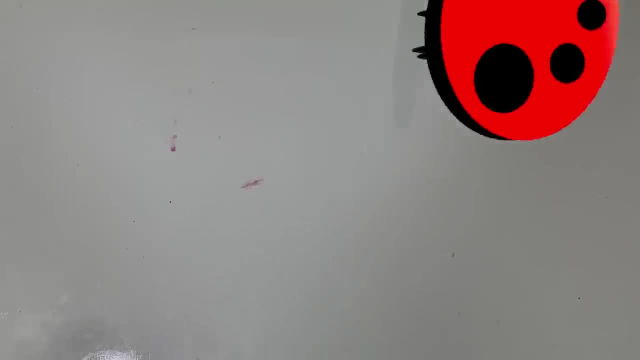 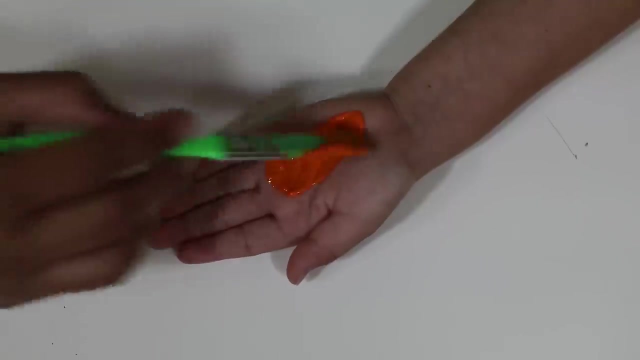 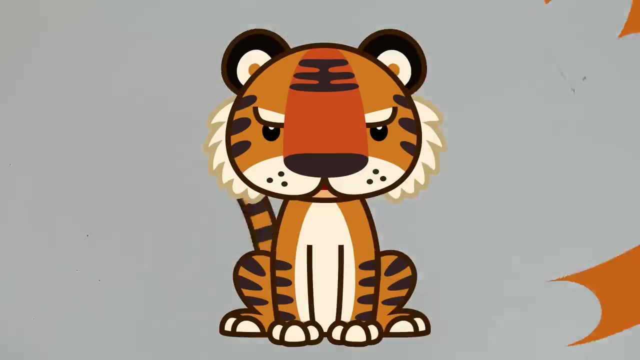 This is red. Now I will paint the ladybug. Wow, the ladybug is red. Wow, The ladybug fly away. Now I will paint my tiger- orange, Orange, Wow, the tiger running away. That's awesome. 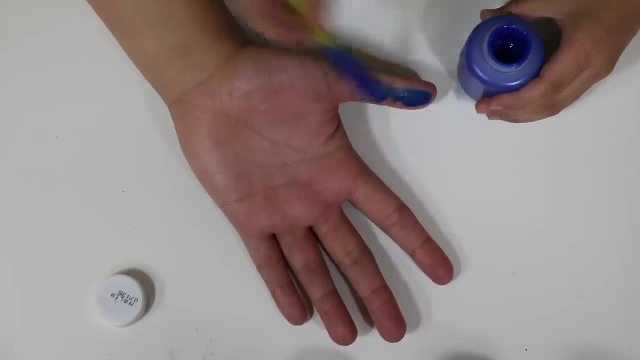 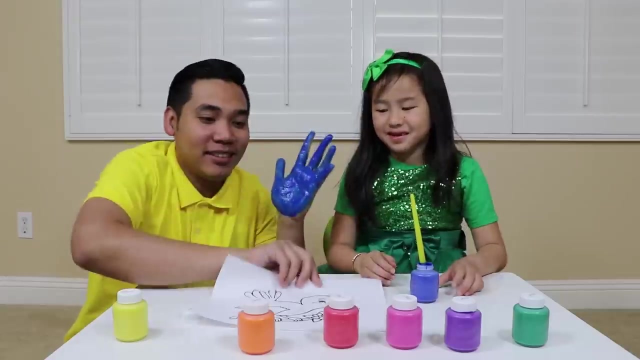 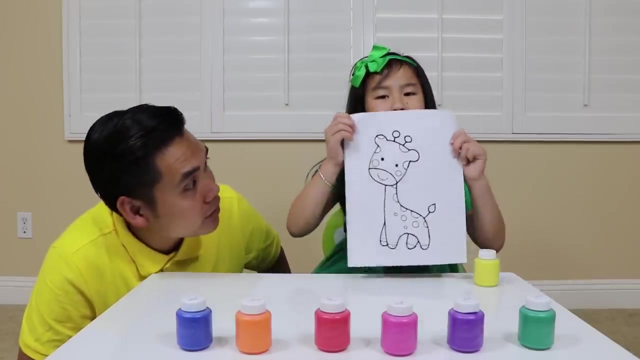 Next, I will paint the bunny. I will paint the bird blue. This is blue. Now I will paint the bird. The bird is blue. Check out the bird guys. Wow, This is a giraffe And I'll paint it yellow. 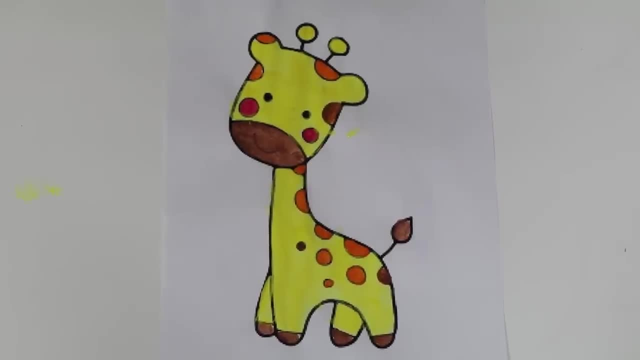 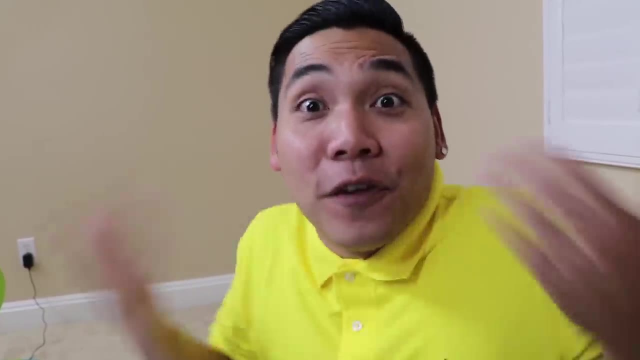 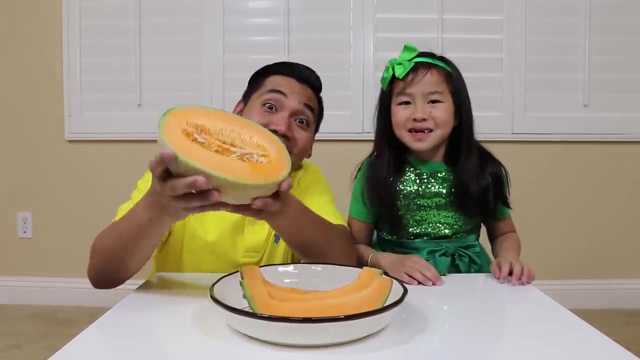 This is the color yellow. Wow, Wow, Wow, The giraffe run away. Next we're going to learn about the fruit and its color. Let's open it, uncle John. Okay, Wow, What fruit is it guys? 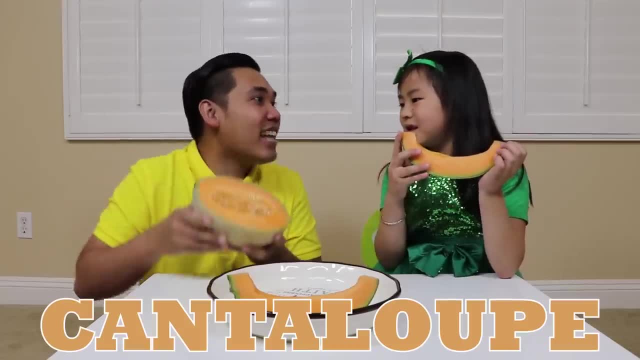 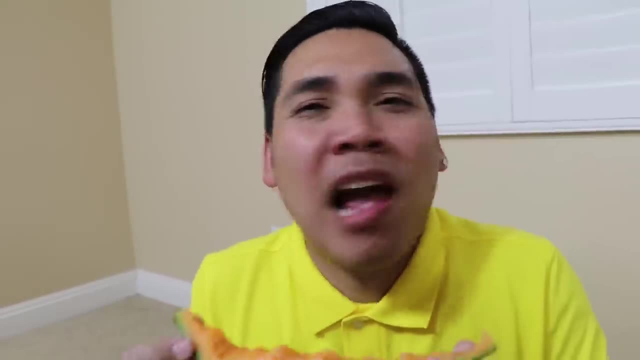 Is it a cantaloupe, uncle John? Good job, Jenny. This is a cantaloupe. Yeah, and it's the color orange. Let's try it. I love cantaloupe. It tastes really good guys. 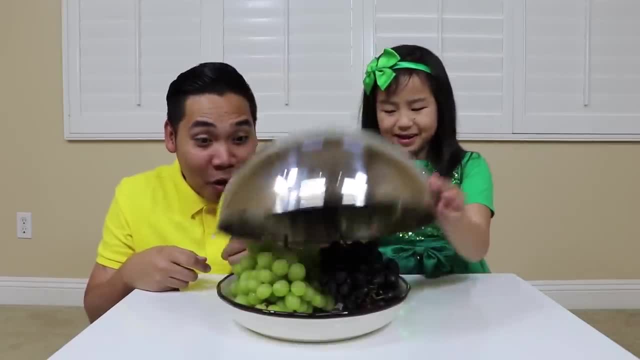 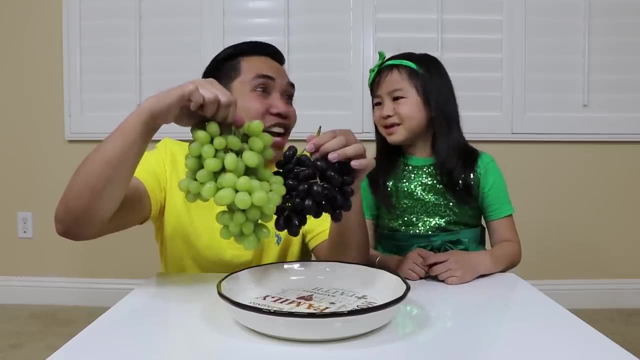 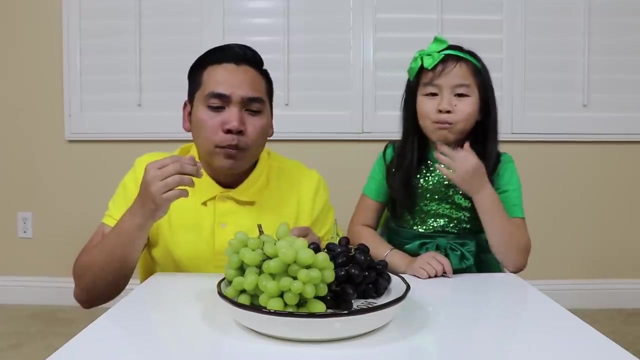 So yummy. Okay, uncle John. Wow, What fruit is it guys? Is it grapes? Yeah, you're right, Jenny, This is the green grape and this is the black grape. Let's try it. Yeah, Wow, it's too soft. 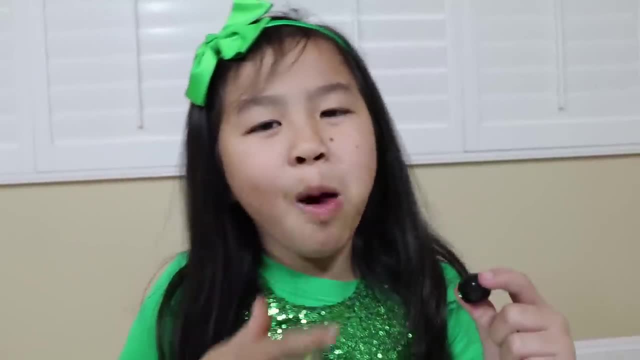 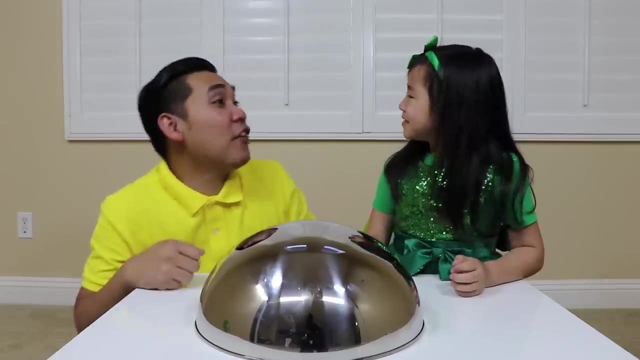 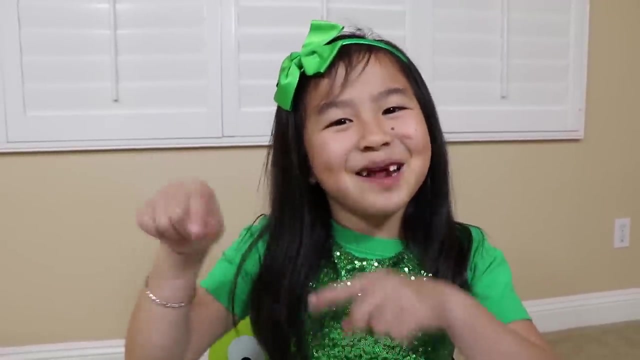 Wow, it tastes so sweet. Let's try the green one, Mmm. Let's try the black one now, Mmm. delicious, Are you ready for the next one? Yeah, Wow, What fruit is it guys? I think it is a green watermelon. 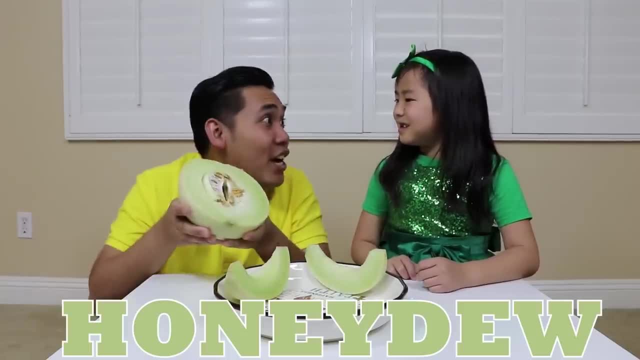 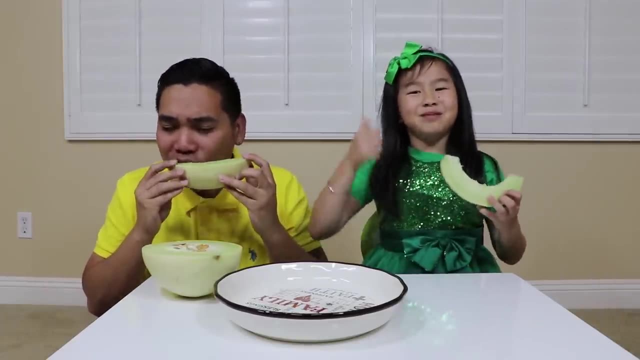 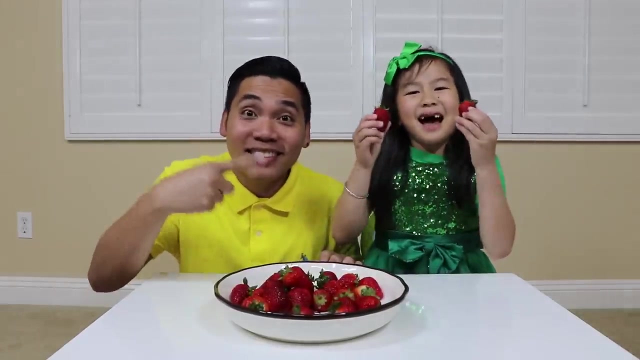 No, it's not a watermelon, It's a honeydew. Let's try it, Mmm, It's too soft and sweet. Yeah, it's so sweet, Mmm, so delicious. Wow, What fruit is this guys? 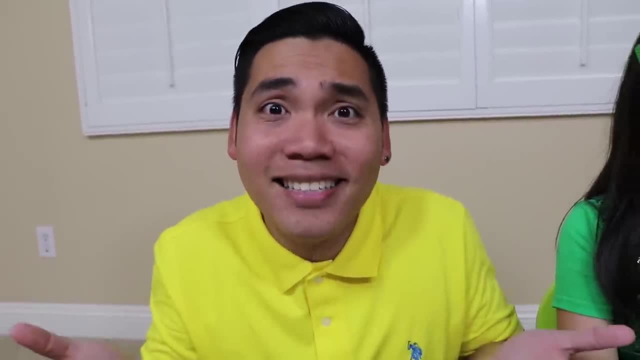 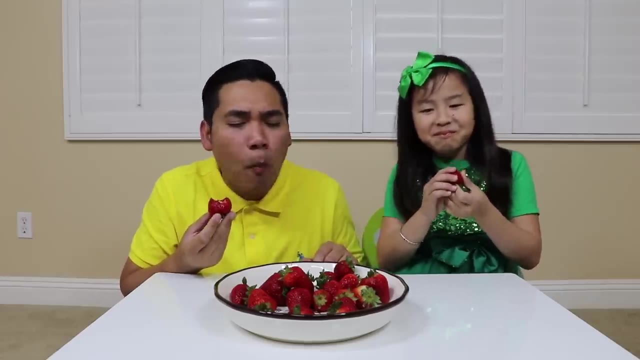 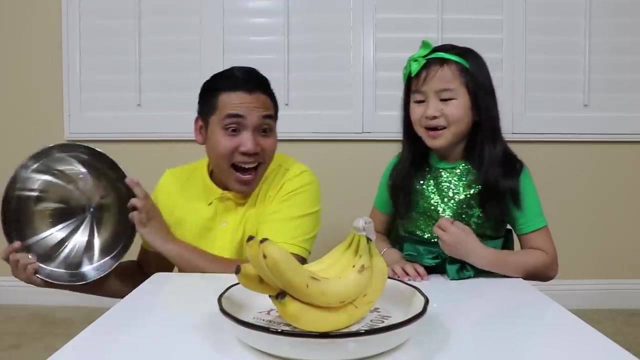 It's red, It must be a strawberry, guys. Yeah, Uncle John, Let's try it. Okay, I will choose a big one. Mmm, Wow, This one is too sour, guys. Jenny, let's open it, Okay. 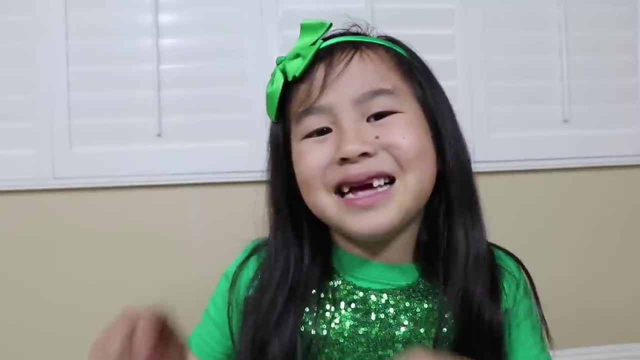 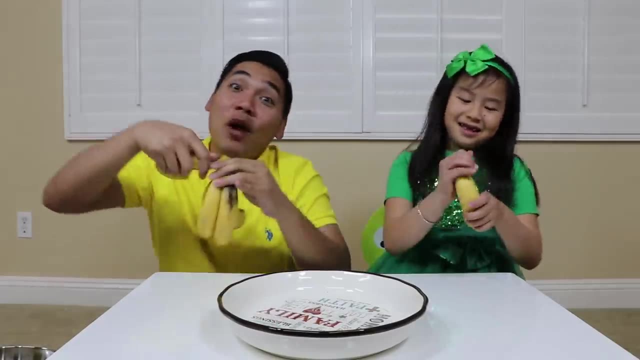 Wow, What fruit is it guys? It's yellow and long, so it's a banana. Good job, Jenny. This is banana. Try one. Okay, I'll try one too. Mmm, It's really tasty guys. 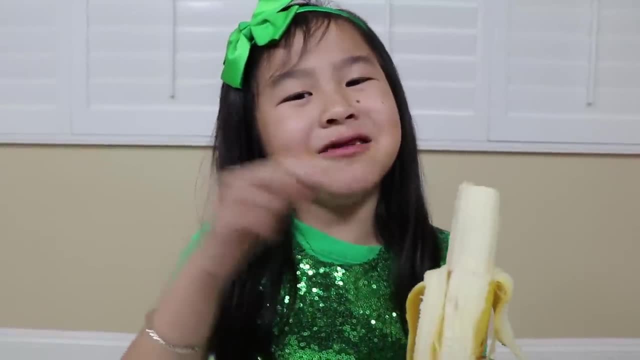 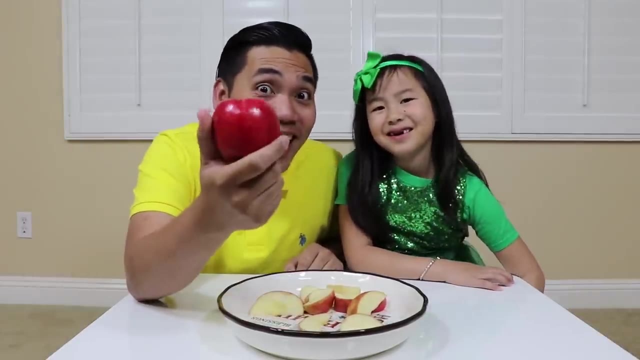 I love it. It's soft and it's easy to eat. Are you ready for the next fruit, Jenny? Yeah, Open it. Wow, Wow, What fruit is it guys? Yeah, it's an apple. Yeah, you right, Jenny. 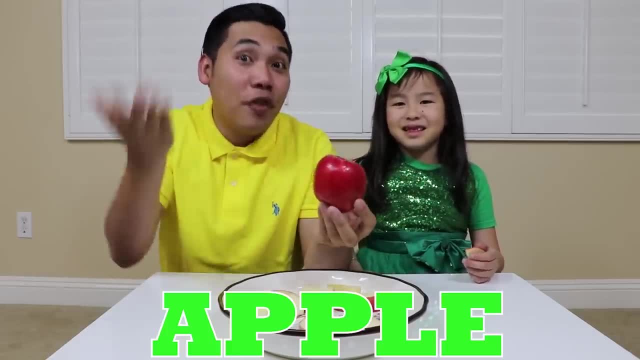 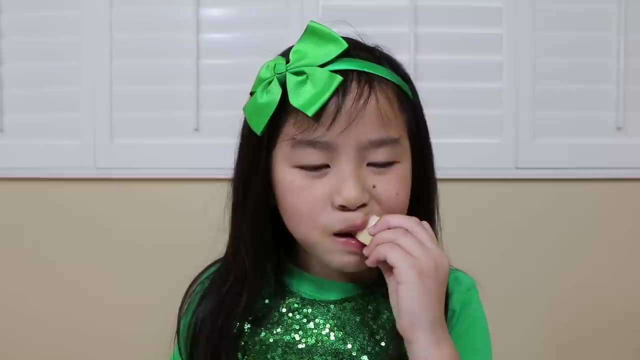 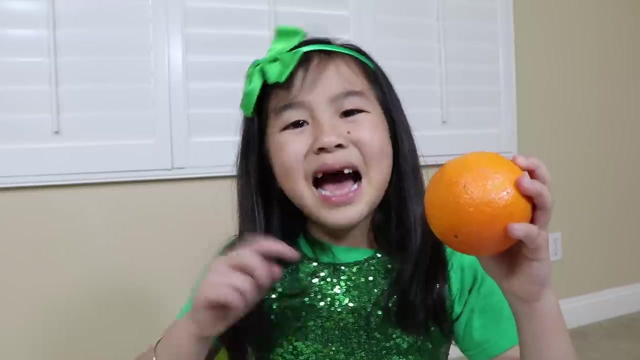 This is apple. Apple has a red. sometimes it has a green and yellow color. Let's try it, Okay, Mmm, So yummy. This is my favorite fruit, Ta-da. What kind of fruit is this, guys? You're right, It's an orange. 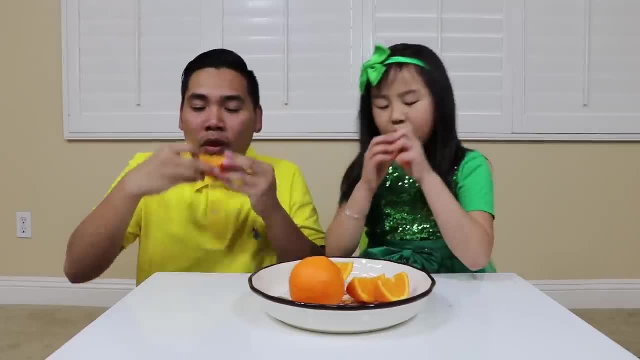 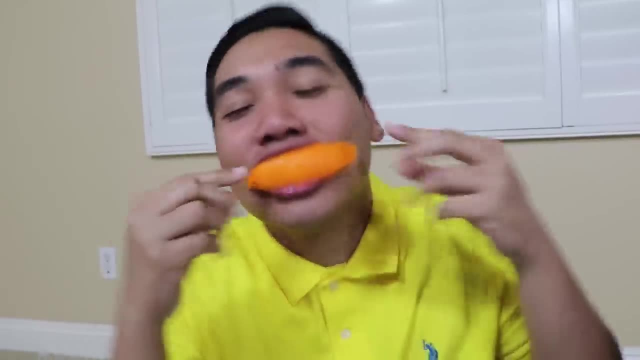 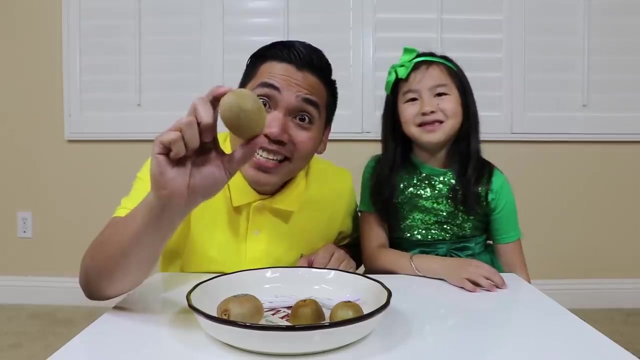 And it's like this color. Let's try it. Okay, Mmm, It's so juicy, Yeah, And sweet too. This is a lot stronger, John. Okay, Open it. Wow, What fruit is it guys? 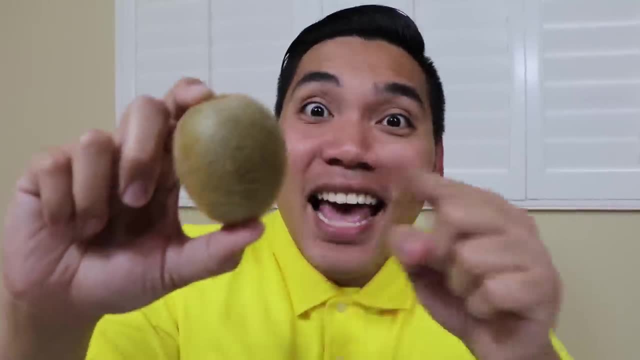 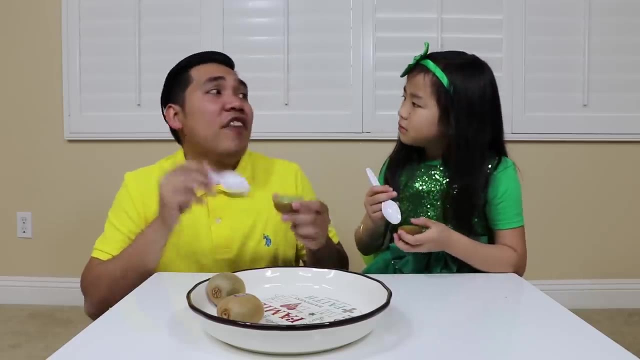 It's a color brown and it's very fuzzy. Yeah, you right, It's a kiwi. Yeah, It's sour like a lemon. Mmm, I know it's sour, but it's very good for your health. What is your favorite fruit guys? 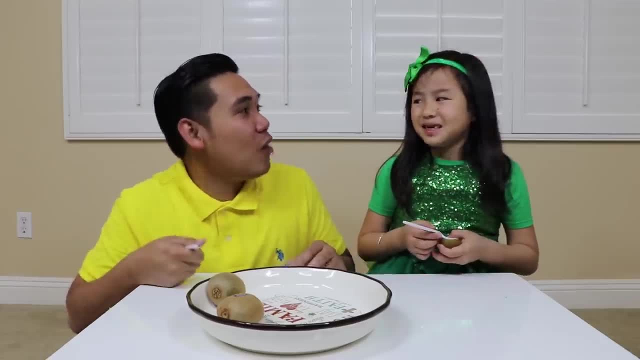 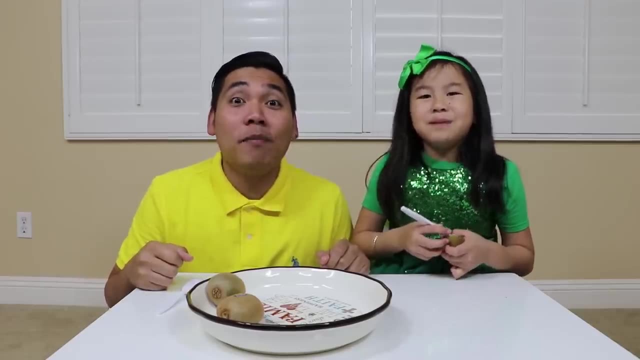 Mine was cantaloupe And mine was apple. How about the color? What's your favorite color? Red, And I love yellow guys. Thank you for watching. Hope you guys enjoy our show. Please remember to subscribe to our channel and click the bell button. 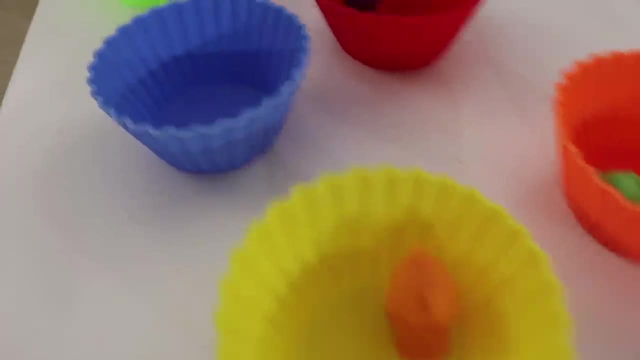 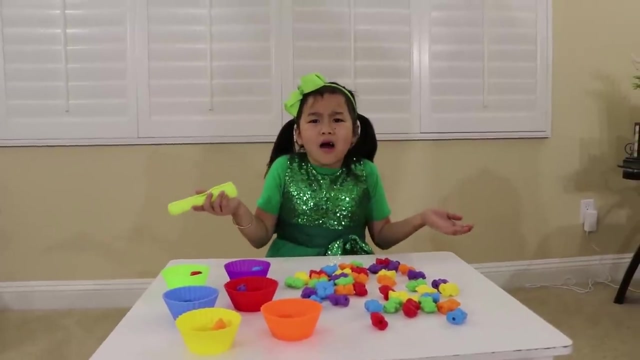 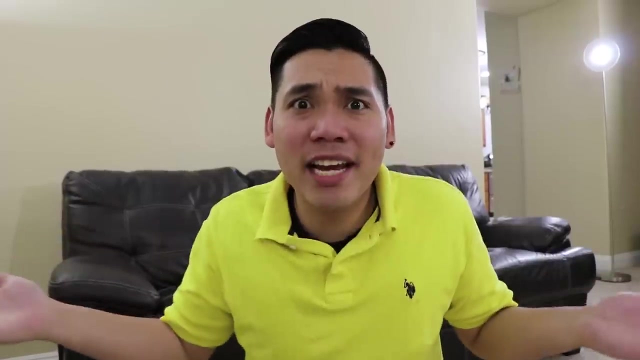 See you next time. Bye. Green, blue, orange. Is that right, guys? Yeah, Huh, I'm wrong. Learning colors is so hard, Hi, Jenny, Hi, Uncle John. What's wrong, Jenny? I tried to learn the colors, but. 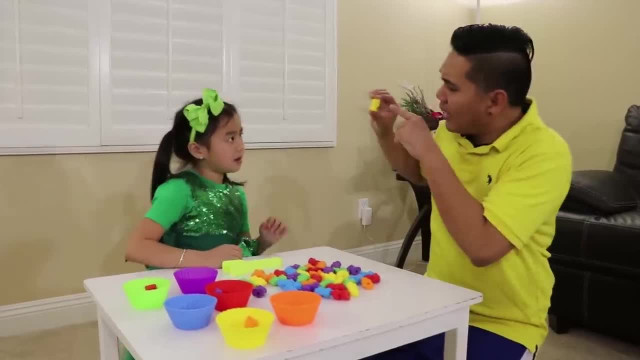 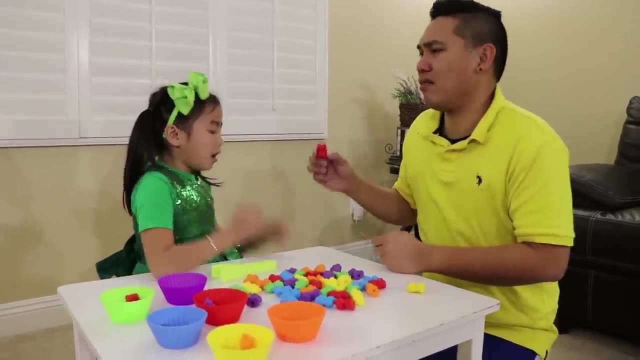 it's too hard, Really. Let me test you. What color is this Orange? No, Jenny, It's yellow. How about this one Green? No, It's red. See, I told you, Uncle John, Learning colors is so hard. 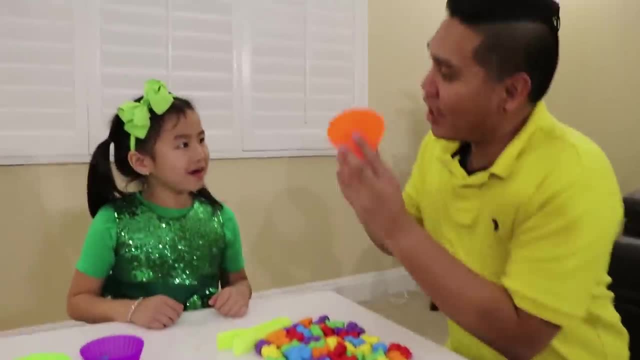 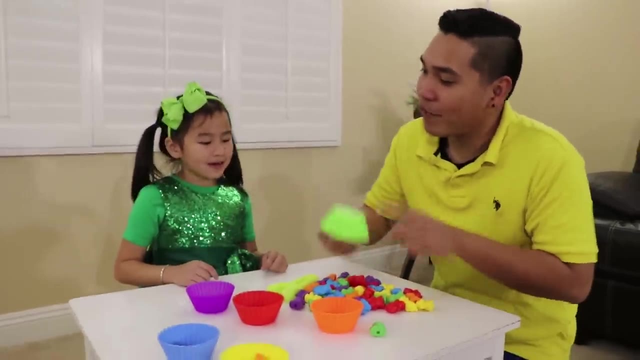 Don't worry, Jenny, I will teach you. Thank you, Look. This is orange, Orange, This is red, Red. This is purple, Purple. This is green, Green, This is blue, Blue And the last one is yellow. 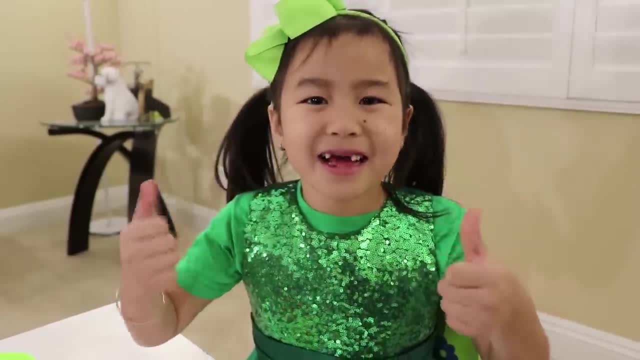 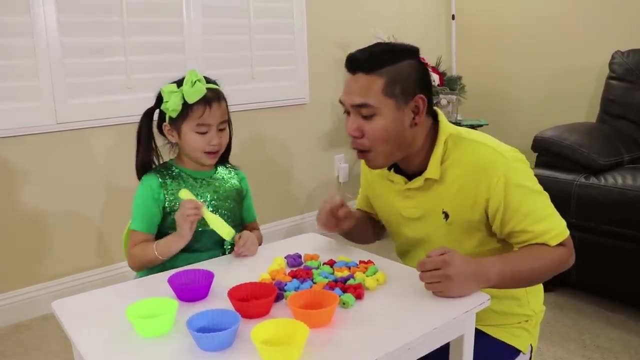 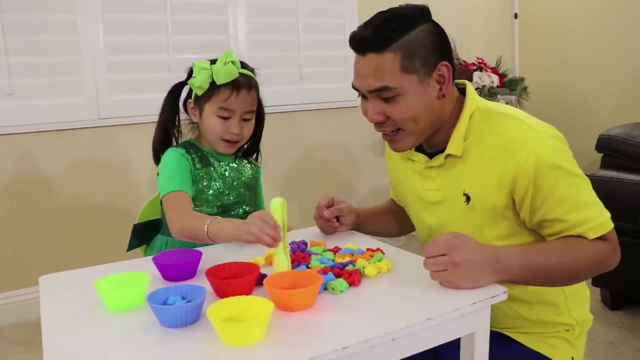 Yellow. See, it's easy, right? Yeah, I think I got it, Uncle John. Okay, Jenny, I will test you. Let's put the red in the red cup. How about purple, Orange, Blue, Green And the last one is yellow. 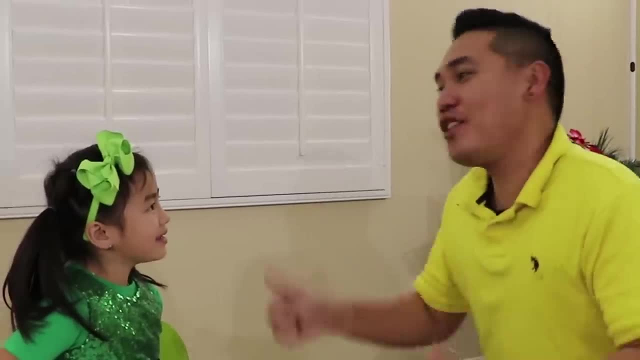 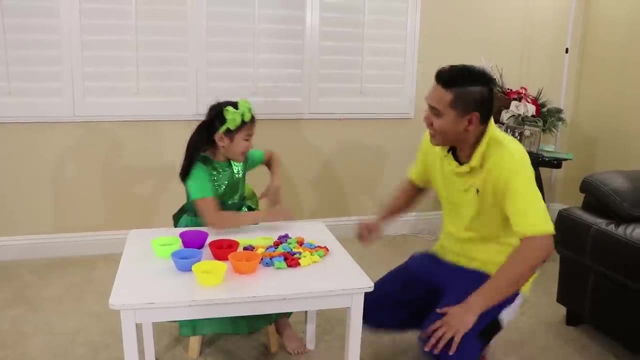 Okay, Wow, Good job. Good job, Jenny. You passed the test. Yay, Now let's go to play the color game. Color game- What's that I'll show you. Follow me. Okay, Let's go. 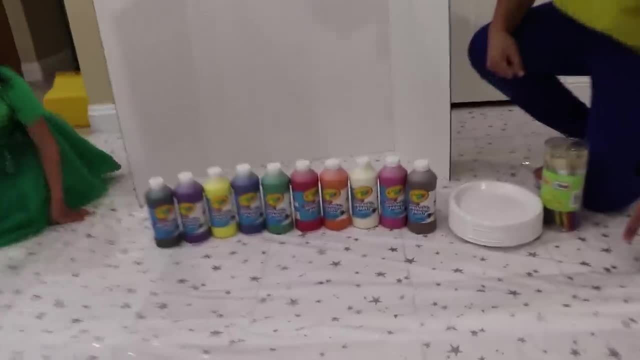 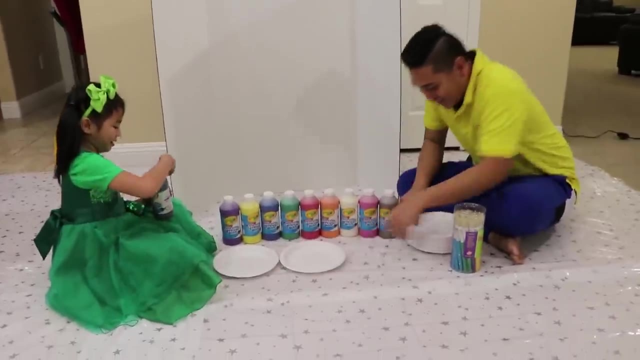 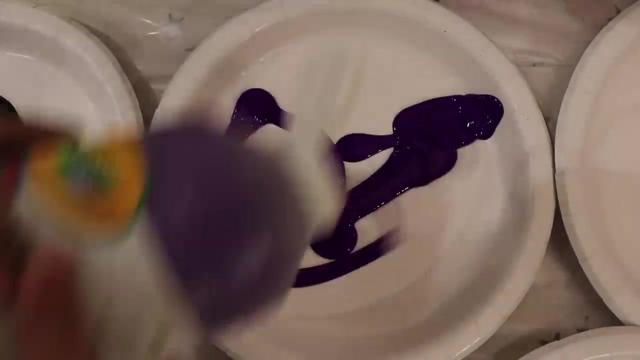 Jenny, check out all the colors. Wow, What's all the color pink? for It will help you learn the colors Here. Put the colors on the plate. Okay, This is black. This is purple. It's magenta Brown. 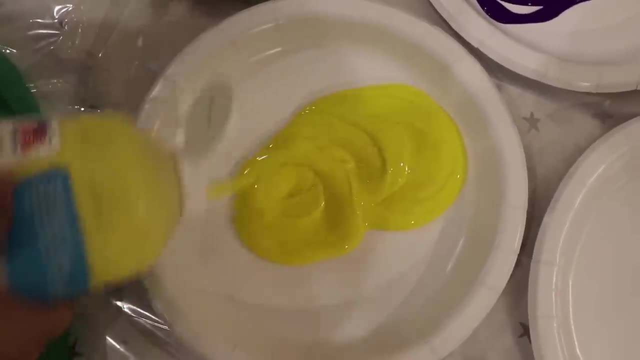 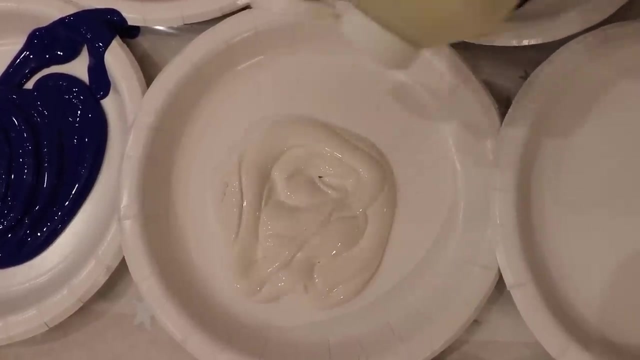 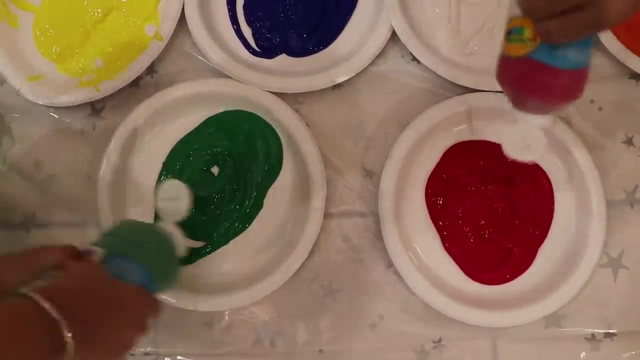 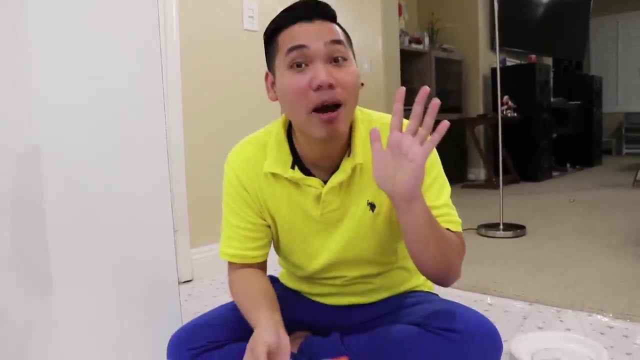 Yellow, Blue, White, Orange, Green And red. What do we do now, Uncle John? Next, you have to pick the brush. Paint your hand with your favorite color. Look at me, I love orange. Wow, That's. 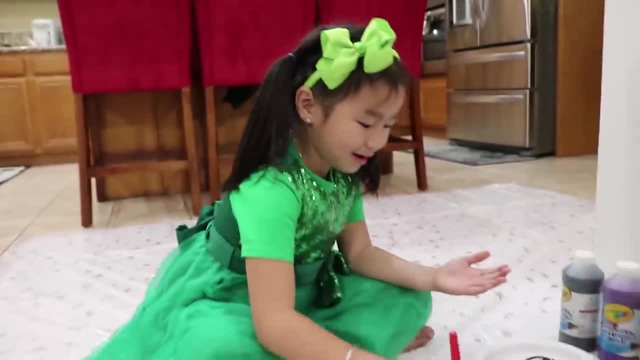 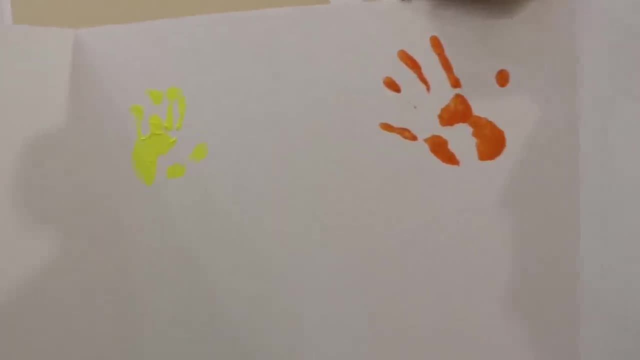 cool, Uncle John. Here's your brush, Jenny, Thank you. Next, you put the hand ring on the wall. Okay, This is orange, This is yellow. That's so cool. Let's do another color, Jenny, Okay. 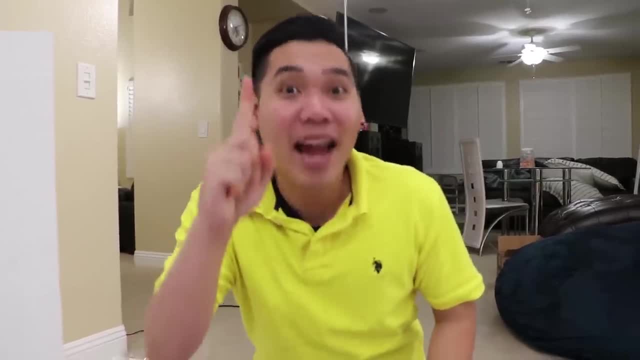 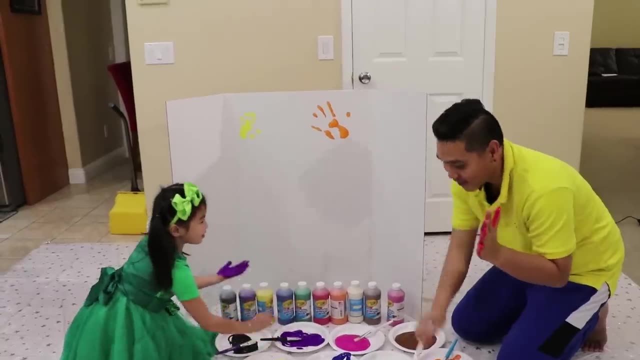 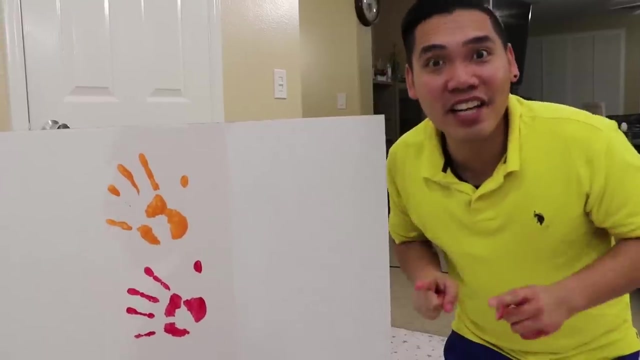 Purple will be awesome, Jenny, I will pick red. Look at me, This is red color. I'm ready, Uncle John. Okay, Let's put on the board Purple, And this is red. Good job, Jenny. Now we try another game. 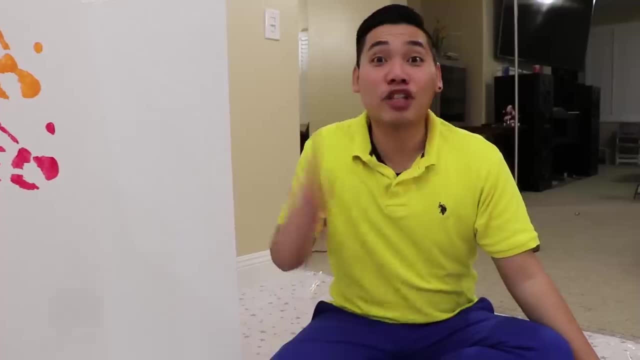 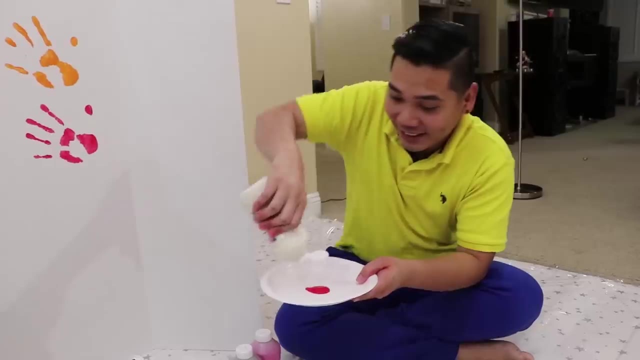 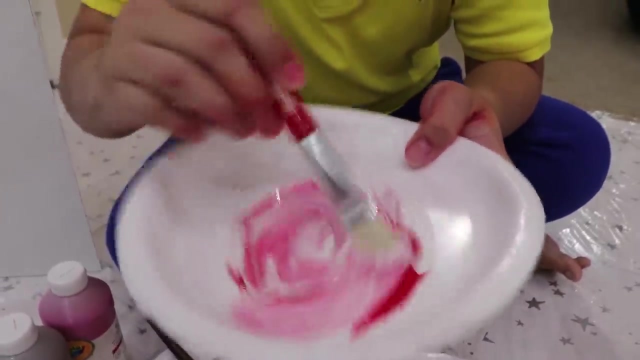 Mixing color game. Mixing color game. What's that I'll show you. First you pick the plate and then pick two colors. I choose red and white. Then you use the brush to mix it up. See what happens. Wow, I wonder.